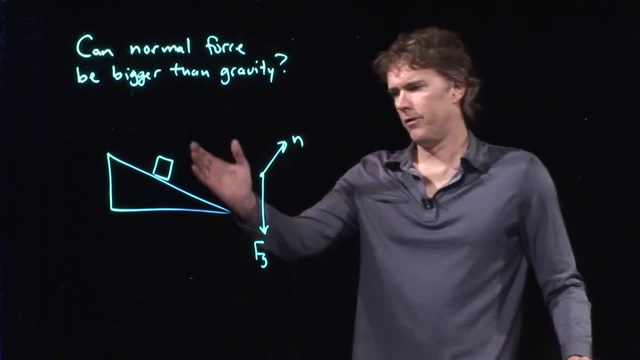 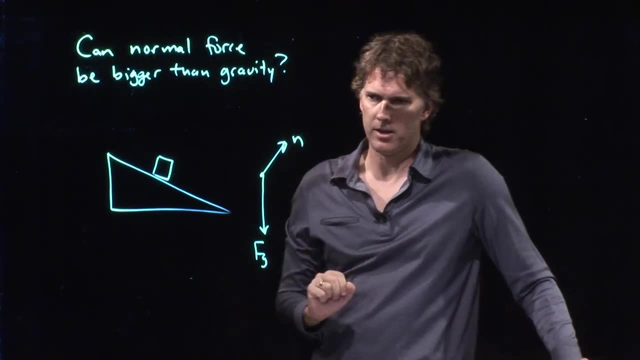 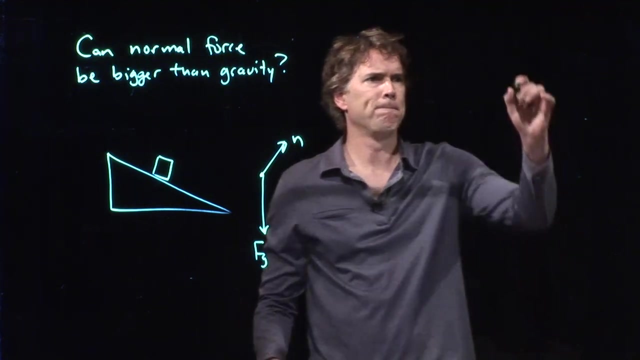 Okay. So if it's equal to gravity at the horizontal- and it gets smaller as I tip it up, that thing is always less than gravity. But can you have a situation where the normal force is, in fact, bigger than gravity? Well, let's think about it. Let's say that we're in an elevator. 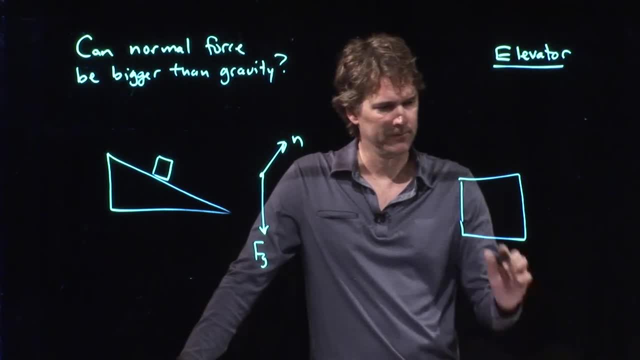 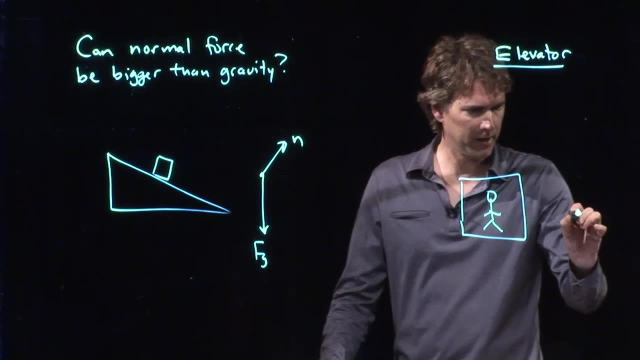 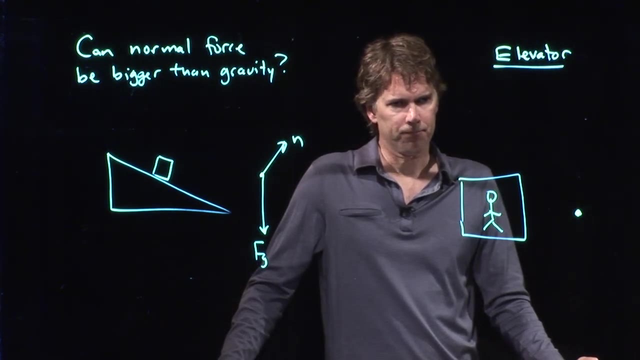 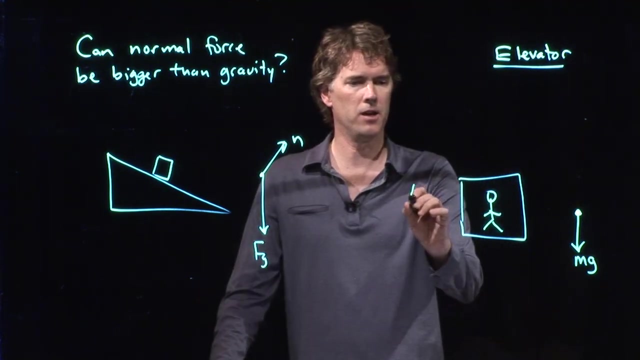 And now you're just standing in the elevator And the elevator is not moving. What are the forces that are acting on you in the elevator, Allie? what do you think? The force of gravity downwards, Force of gravity M-G? Okay, And you are in the elevator and the whole elevator is at rest. What else, Allie? 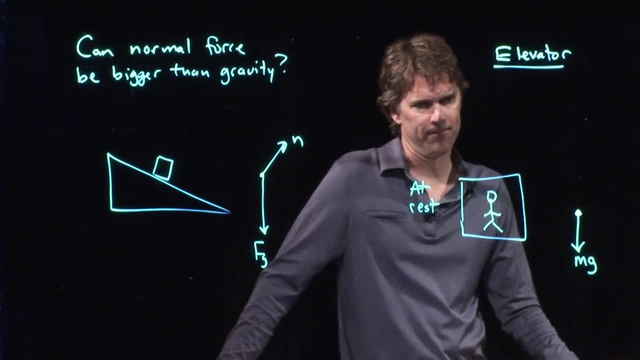 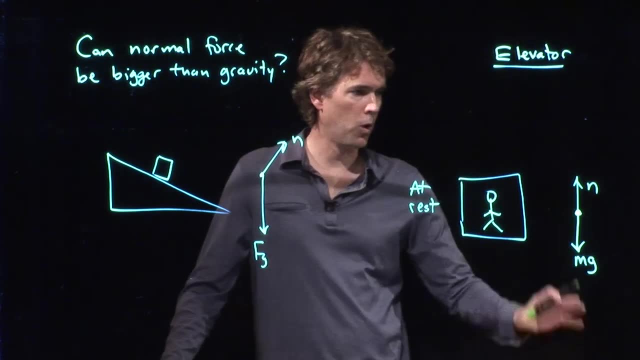 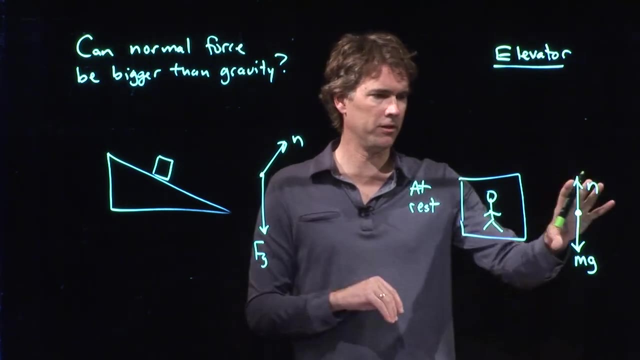 The normal force? Which way? Opposite of gravity? Okay, How long? Same length, Same length, Exactly right. Normal force is the floor pushing up on me, Gravity is pulling me down. Those exactly balance out. if I'm at rest, Good, But now let's change. 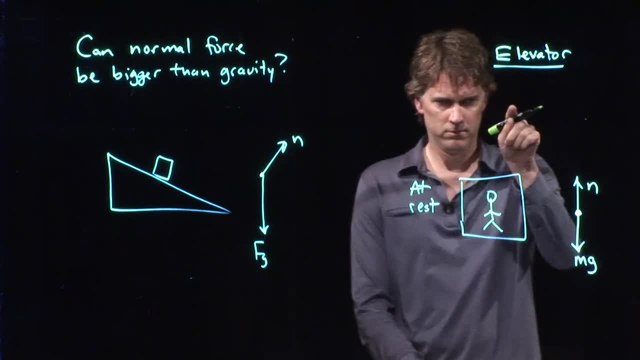 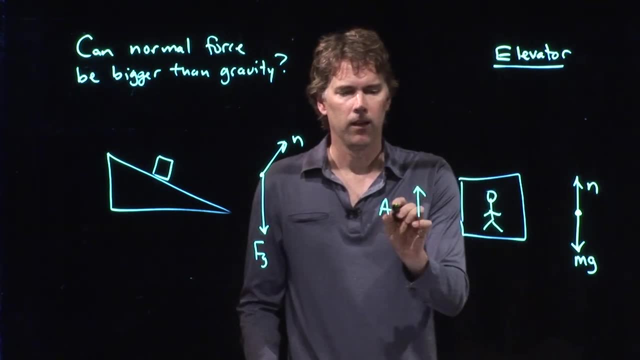 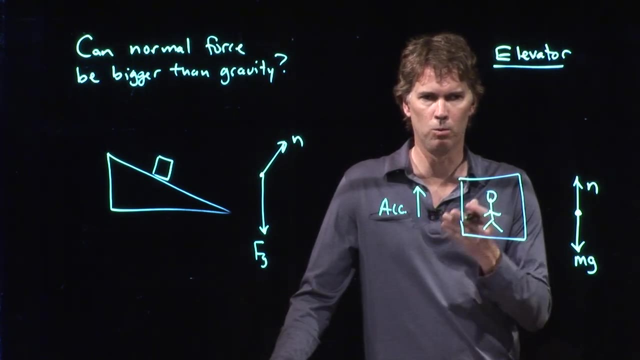 the picture slightly. Let's say that we push the floor number six button, trying to get up to the top of PS1. And so the elevator is at rest. And now we're in the elevator, And so the elevator is in fact accelerating upward. Okay, When the elevator first starts moving upward, you're all. 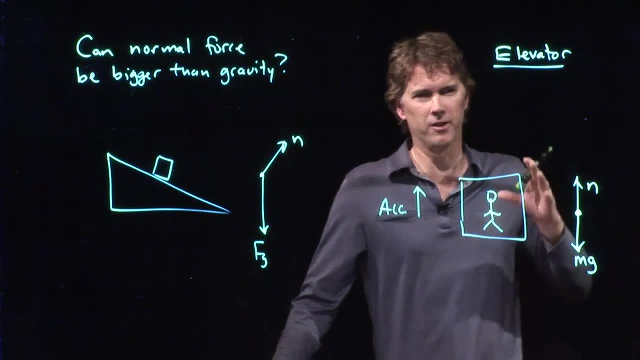 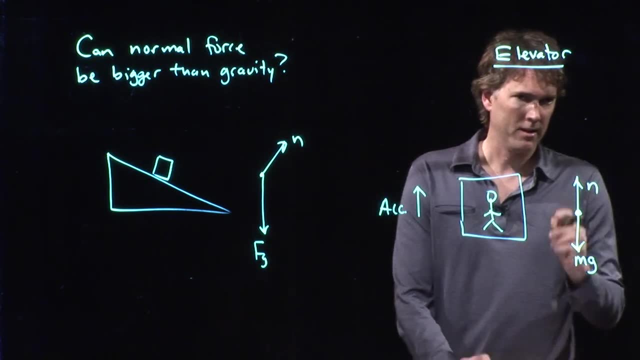 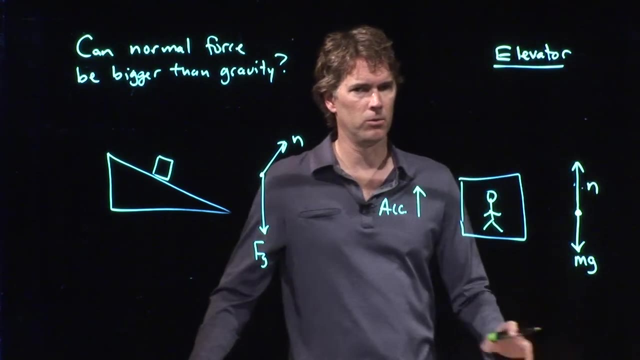 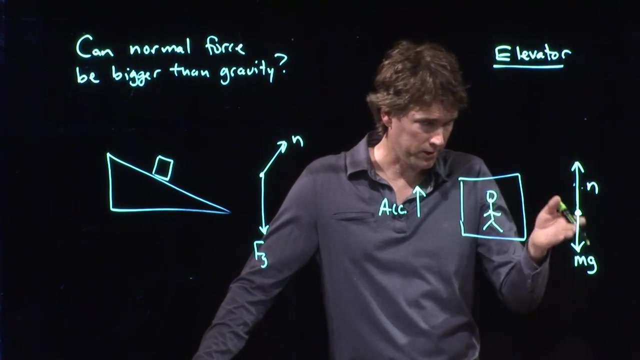 familiar with this. What do you feel? Do you feel lighter or do you feel heavier? Heavier Right, And in fact, the normal force is now bigger than gravity when it's accelerating upwards. Okay, That floor is pushing up on you harder than gravity is pulling down on you, And so you feel a. 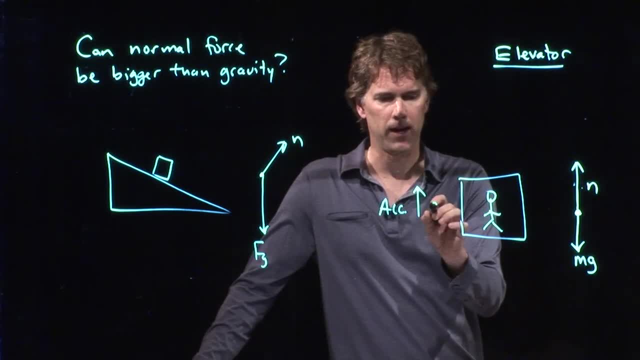 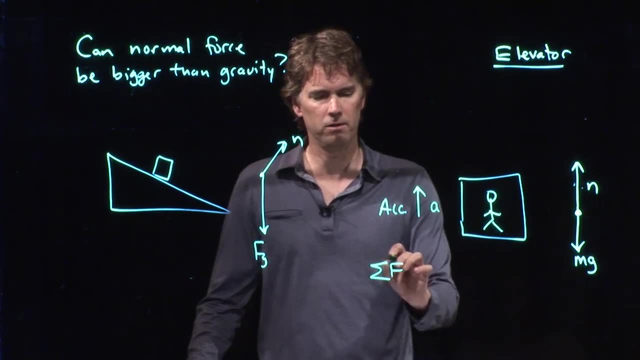 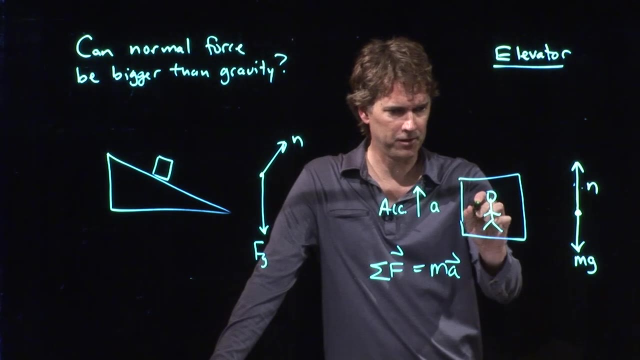 little heavier. How do we see this mathematically? Well, we say that this thing is accelerating upwards with A. What we know is Newton's second law says the sum of the forces is equal to the mass times acceleration. We are mass m. This is a vector equation, And so we can. 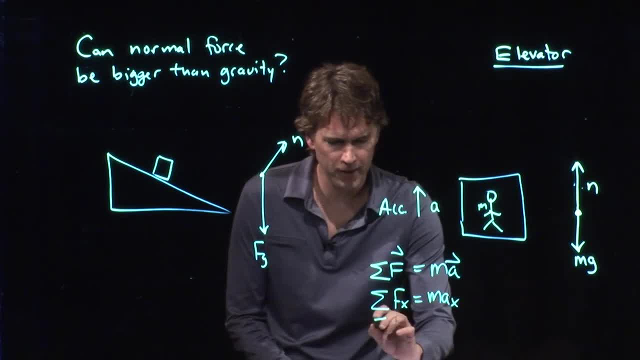 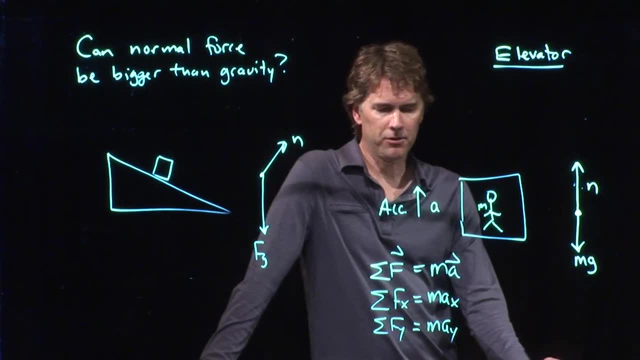 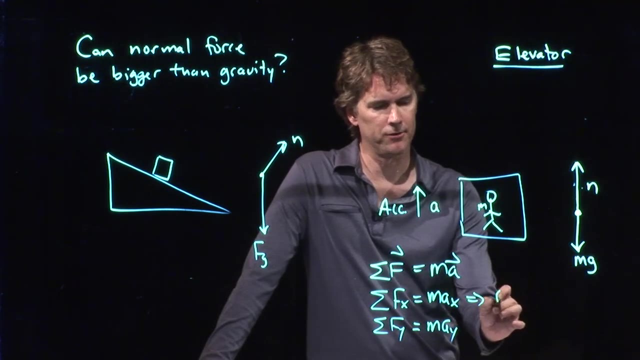 write two equations, one for the x direction, one for the y direction. But the x direction doesn't really tell us anything. Right? There's no forces in the x direction. We're not moving left or right. Zero equals zero, Good. 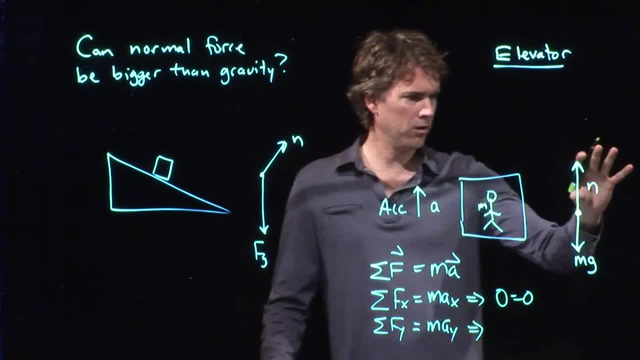 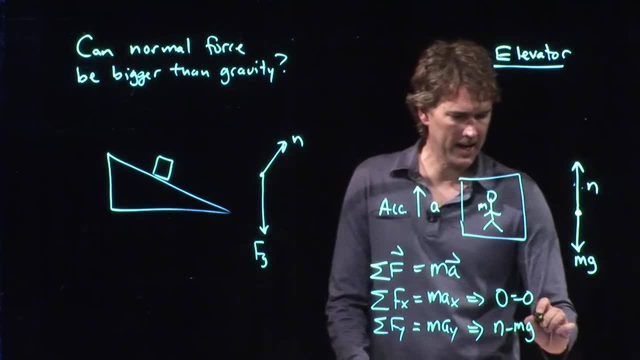 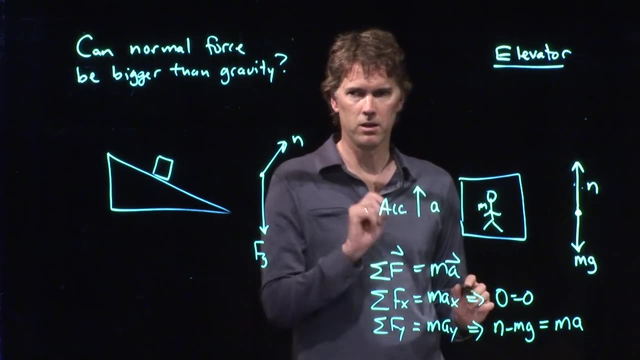 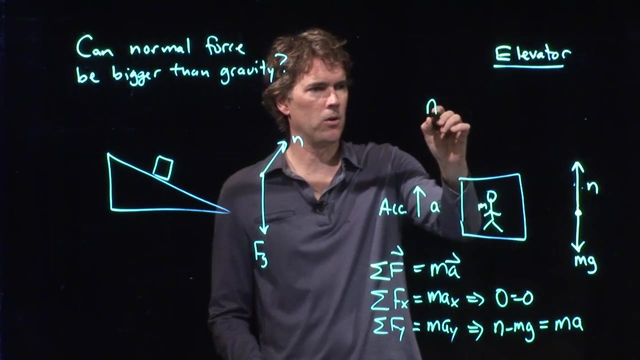 What about in the y direction? Well, here are the forces: N is going up, Mg is going down. All of that has to be equal to the mass times, the acceleration upward in the elevator. And now look at this equation. I can solve this very quickly And I get normal. force is equal to ma plus mg And I get normal. 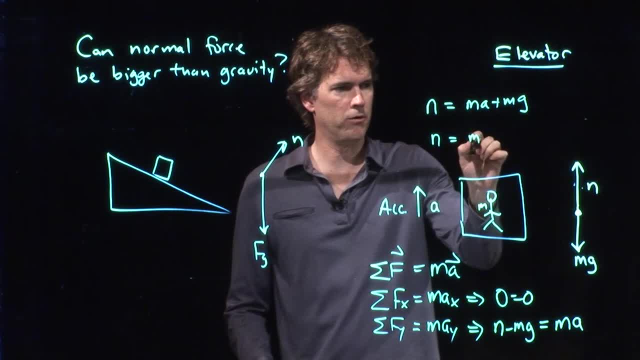 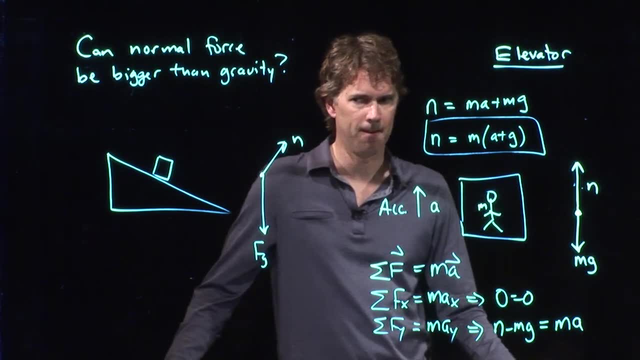 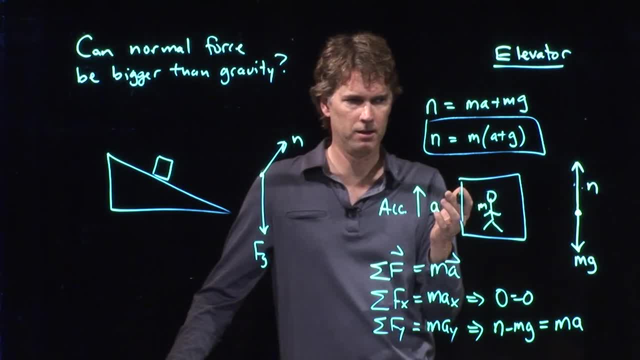 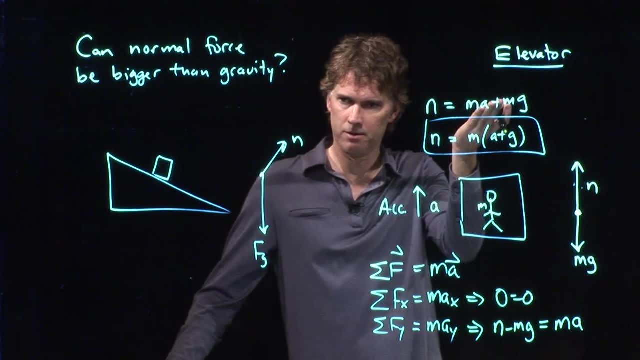 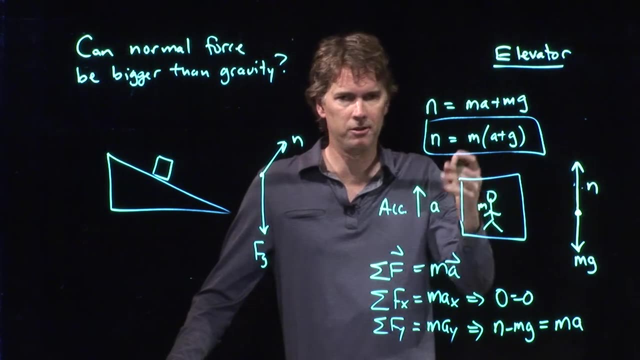 force is equal to m times a plus g. The normal force can absolutely be bigger than gravity, but only in the case where you are accelerating, in this case accelerating upward. The bigger that acceleration, the bigger the normal force is upward. If it's zero, obviously we go back to 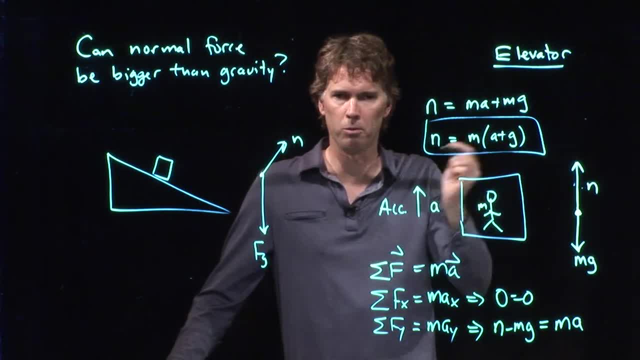 Obviously we go back to the case where the normal force is just mg. But let's look at the other case. Let's say you're in this elevator and all of a sudden the cord gets cut right And you are in free fall. 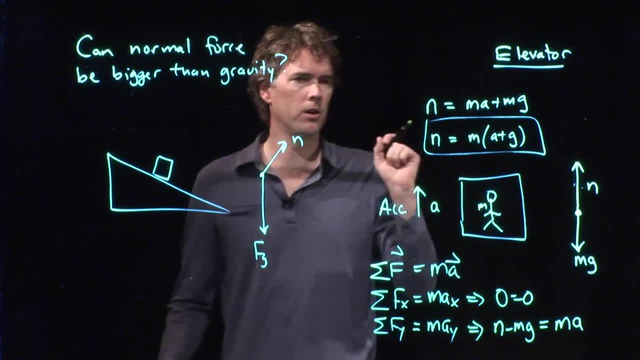 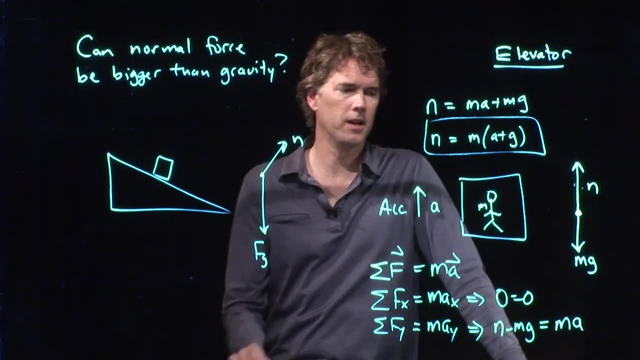 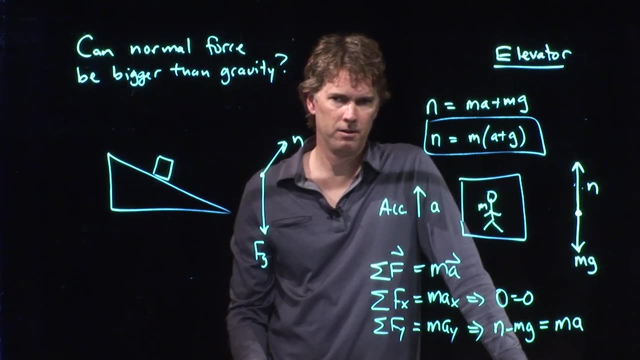 If you are in free fall, what is your acceleration? What was your name? again Anthony, Anthony. What do you think? What's the acceleration if the cable gets cut? It's 9.8 meters per second. Okay, Also known as negative g, right? 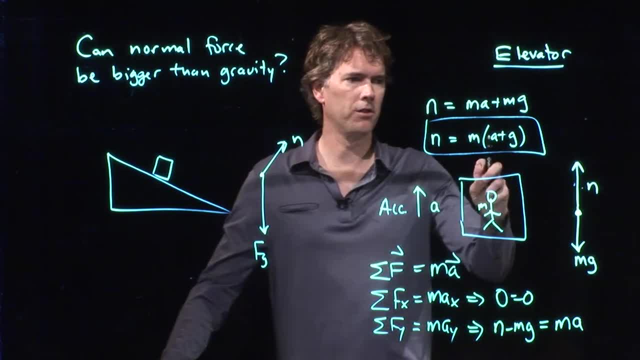 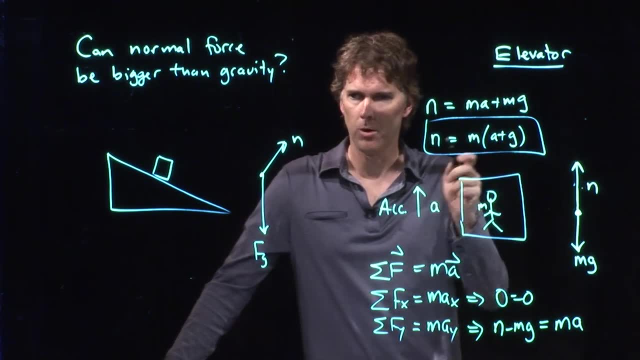 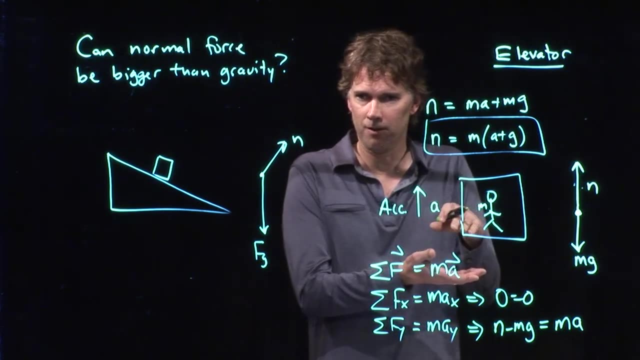 So look what happens If I put a negative g in here. what does the normal force become? Well, it's mass times negative g plus g, It's zero. The normal force is zero, And if you're in free fall, you're not touching the ground anymore, right? 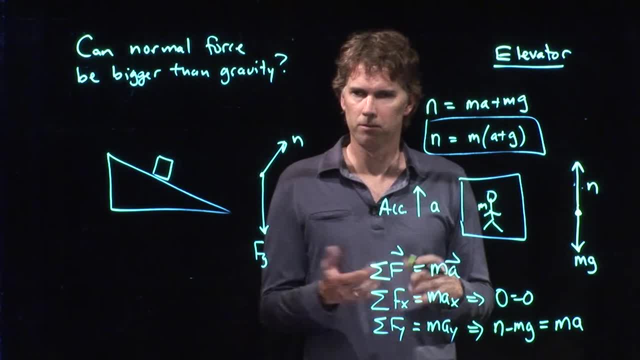 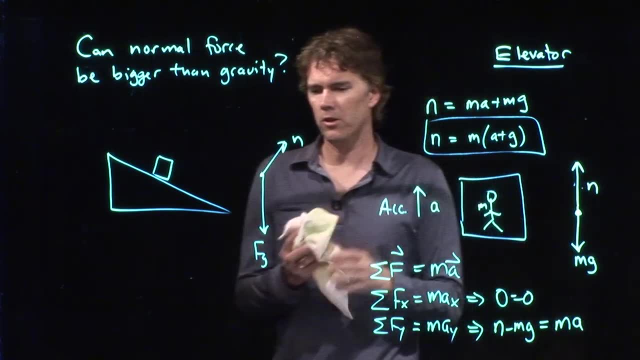 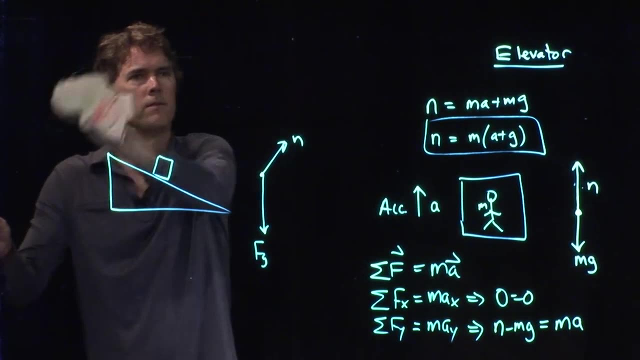 You're floating about in the middle of the elevator, You're probably screaming rather loudly, but okay, The normal force is in fact zero. So this is a good segue into something called weight. Yeah, Anthony, So when you're accelerating, you know I mean eventually on Earth you'll hit ground. 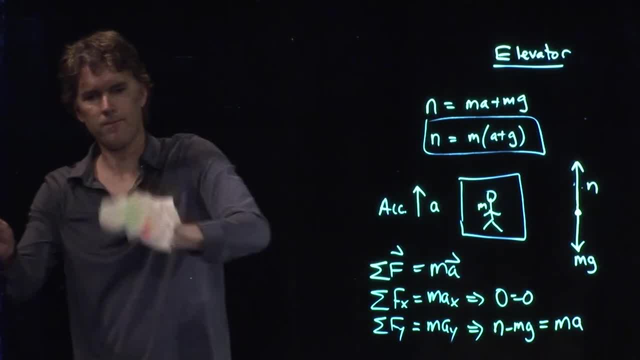 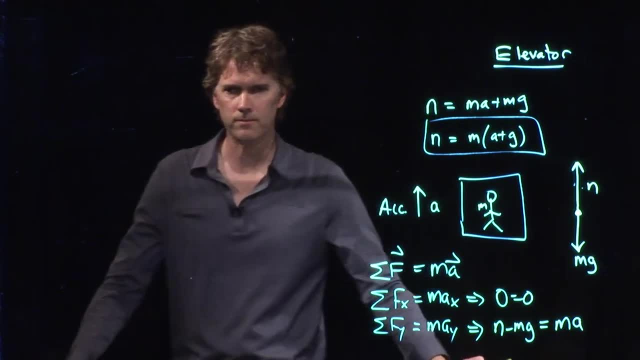 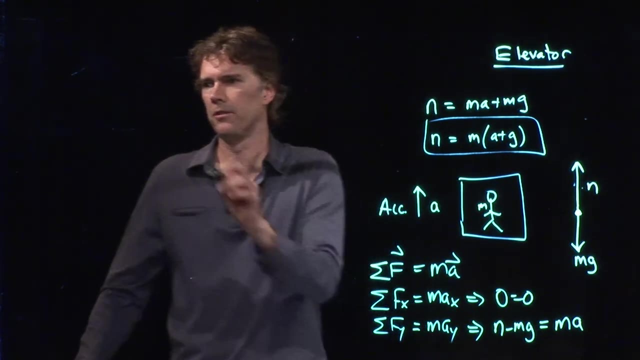 So, but if there was, I don't know if you could go further into the ground or dig a big hole- would you continue to? what would your ultimate velocity be? Would it be infinite? Okay, Excellent question. So the question is the following: 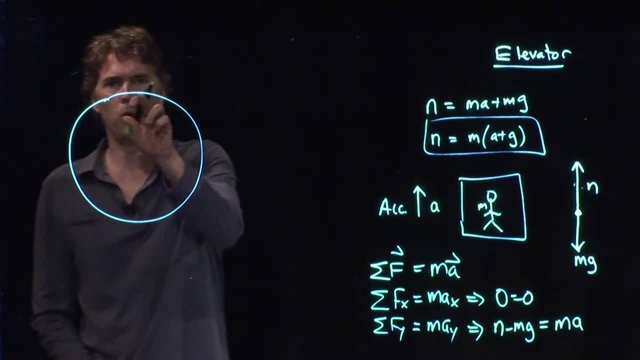 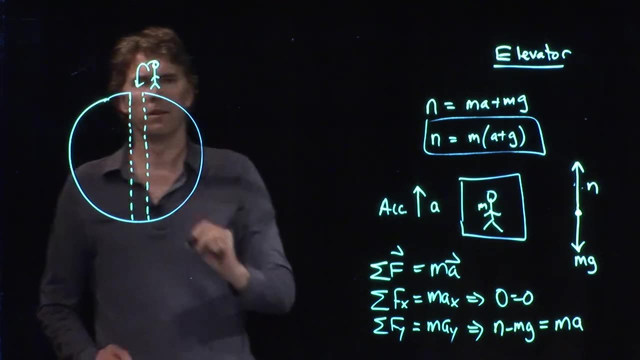 Let's say we start with the Earth and I'm going to dig a big hole in my Earth. okay, Let's dig a really big hole such that it goes all the way through the Earth, And now I'm going to stand here and I'm going to jump into the hole. okay, 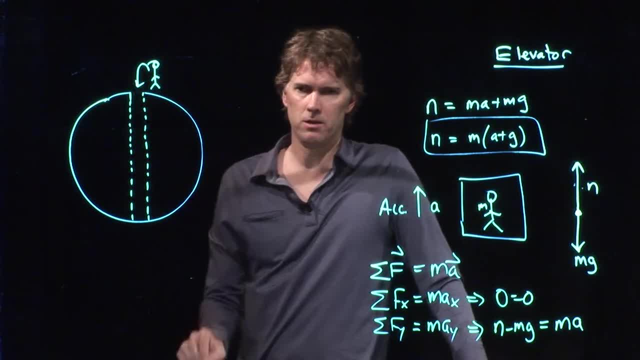 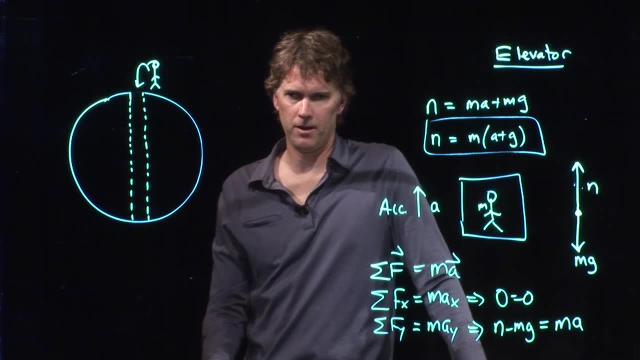 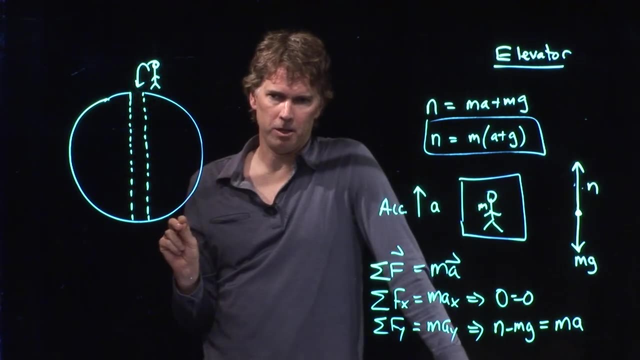 When I jump into the hole? what is my area? What is my acceleration initially? Nine point eight meters per second. Yeah, Negative nine point eight meters per second squared. And if I ignore air resistance, then if I accelerated at negative nine point eight meters, 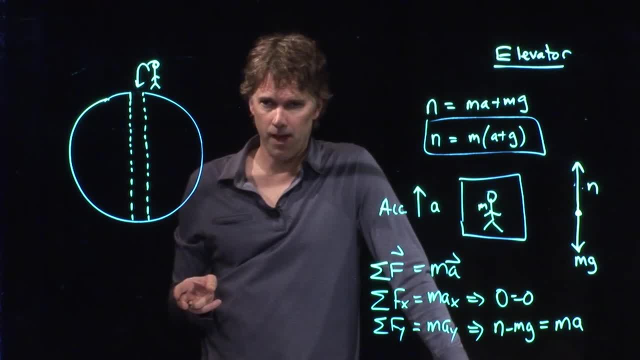 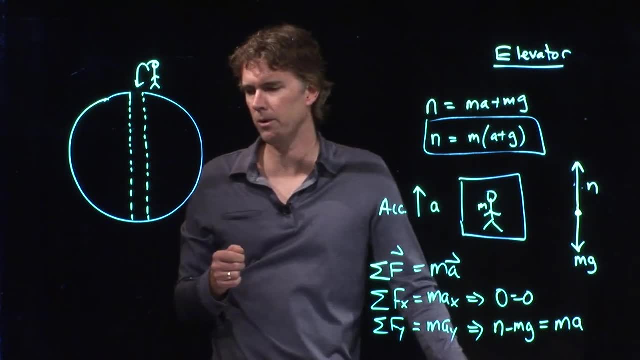 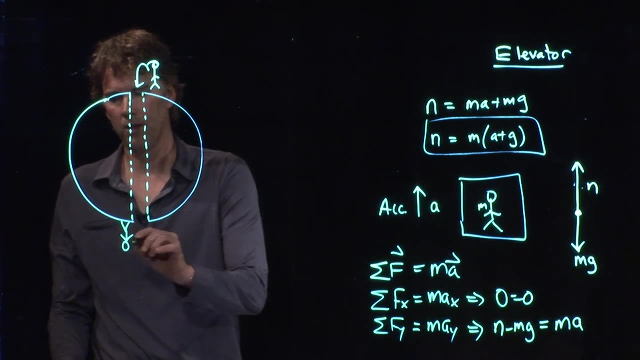 per second squared. if I did that forever, then I would reach infinite speed, But we know that you can't do that forever, right? Why do we know that? Because somebody else That's standing on the other side of the Earth. if they jump in, are they going to? 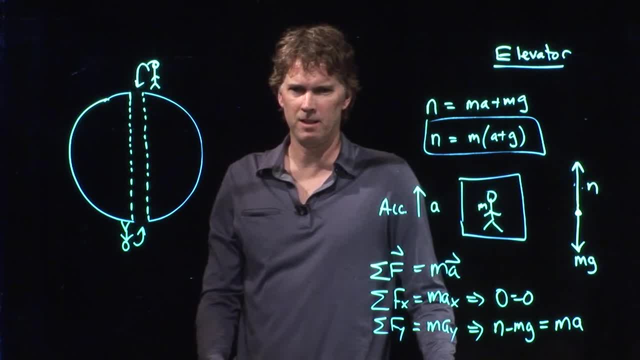 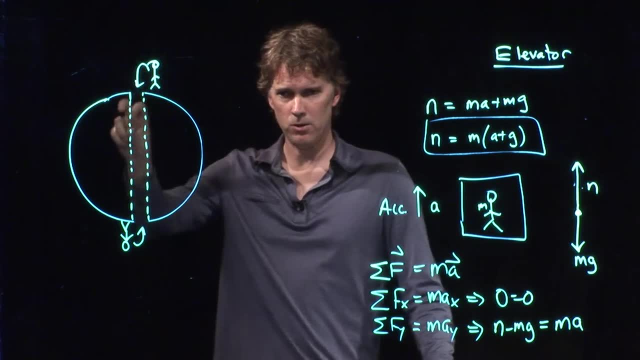 come flying out the top of that tube on the other side. That doesn't really make sense, because this problem has to be symmetric. Whatever I do, if I jump in and start from rest, it should be the exact same as the other person that's jumping in and start from rest. 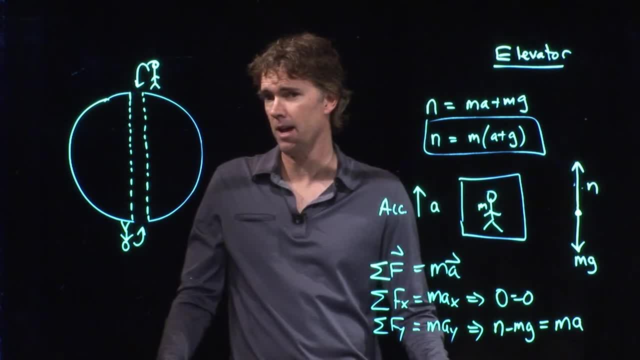 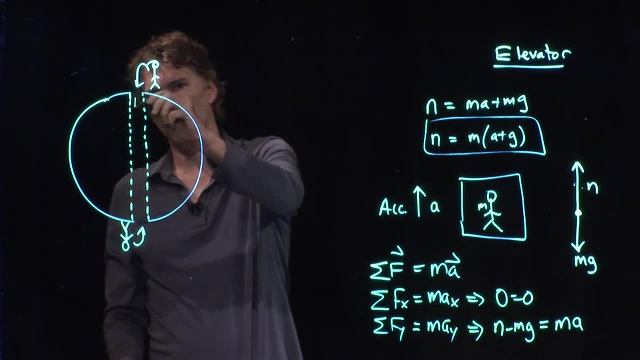 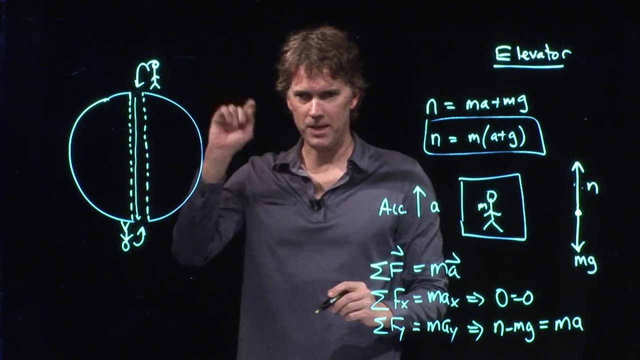 That motion should be the same, And so what is in fact going to happen is the following: With something like the Earth, it's sort of interesting. The person that jumps in speeds all the way through the Earth to the other side just comes up, takes a little peek out the hole and then flies back in and does it again.